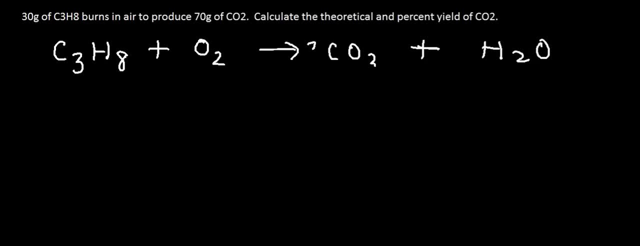 carbon atoms. first, We have three carbons on the left, so we're going to put in three in front of CO2.. Next, we're going to balance the hydrogen atoms. so we have eight on the left, two on the right and we know four times two is eight. And then, finally, we need to balance. 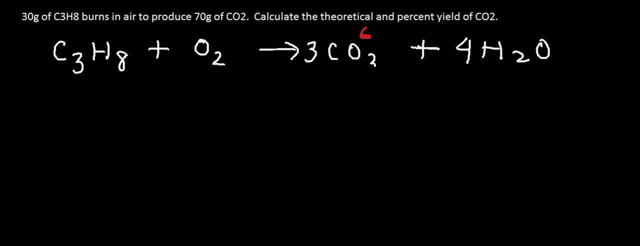 the oxygen atoms. We have six oxygen atoms in the three CO2 molecules, four on the right from H2O. that's 10,. 10, divided by two is five, so we need to put a five in front of O2.. So now let's consider how we're going to balance the questions. If you can, please put them in the 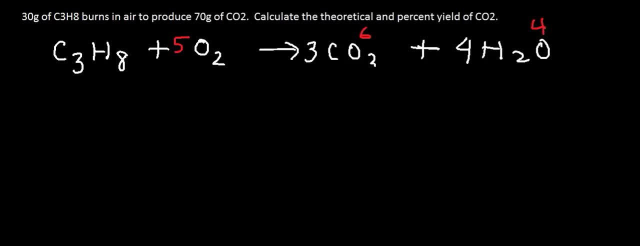 the reaction is balanced. Okay, let's make a list of what we know. We have 30 grams of propane. Now it's burned in air, so we can assume that we have an excess amount of oxygen. Whenever you have two reactants, you need to identify what's the limiting reactant and 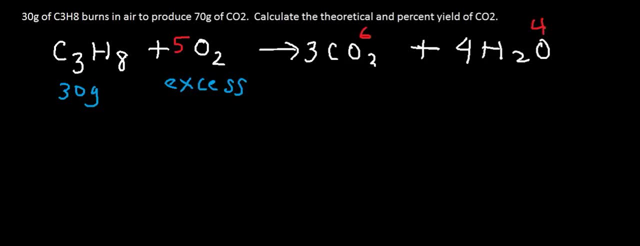 what's the excess reactant? You always want to use the limiting reactant to calculate your theoretical and percent yield, never the excess reactant. Now the equation for percent yield: it is the actual yield divided by the theoretical yield times 100%. So you 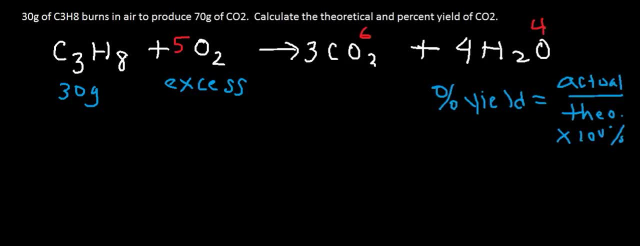 need to know the difference between the actual and the theoretical yield. The theoretical yield is what you calculate. It's the maximum amount of product that you can get. So if your reaction is 100% efficient, you know the amount that you get is the theoretical. 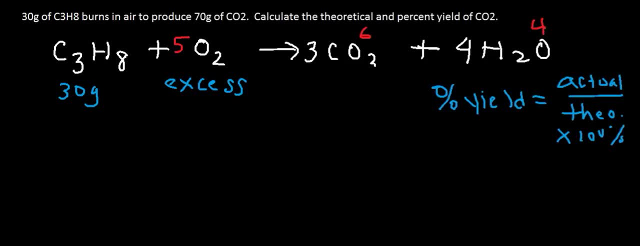 yield In actuality. You know you never get 100% yield. It could be 80%, 70%. you know it's never perfect. The actual amount that you get in a reaction, that's your actual yield. So the actual yield: 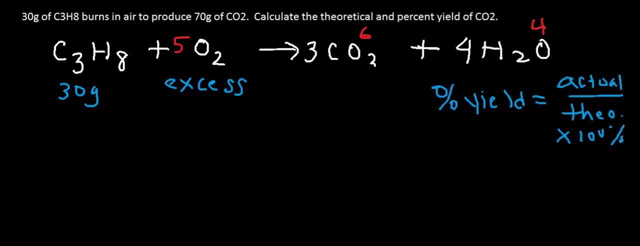 is usually given to you in a problem, unless they want you to solve for it, And the actual yield usually is the grams of product. You see how we want to find the percent yield of CO2? That means that we need to use the actual yield of CO2 and the theoretical yield. 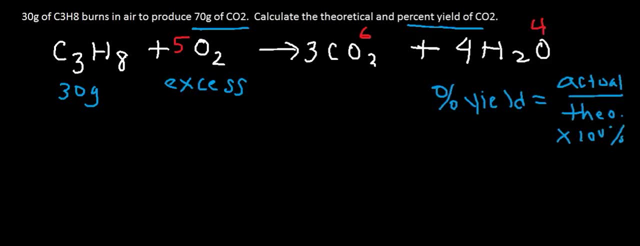 They gave us the actual yield. They said: you know, we, you know, 70 grams of carbon dioxide was produced. That's how much we actually got in the experiment. So we know the actual yield. What we don't know: 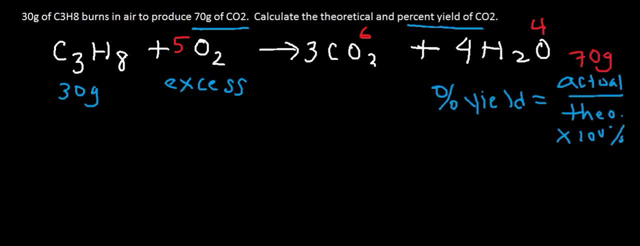 is the theoretical yield, the most that we can get from the experiment. So let's calculate the theoretical yield, the maximum amount of CO2 that is possible to get. So we're going to start with the 30 grams of propane. We're going to see how many grams of CO2 can. 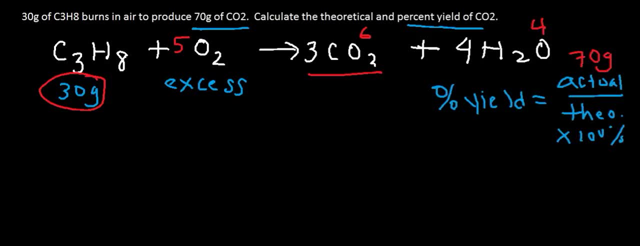 be produced at most from 30 grams of C3H. So let's start with 30 grams of C3H8.. The first step is to convert to moles using molar ratio. So the molar mass of C3H8, which we get from the periodic table, it's about 44. 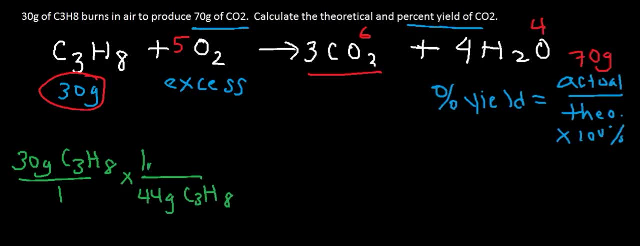 grams per 1 mole. You know carbon has an atomic weight of 12.. So 12 times 3 is 36.. Hydrogen is about 1, and there's 8 of them. So 8 plus 36, you get 8 plus 36.. So you: 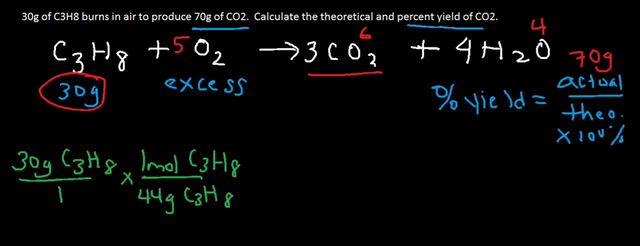 get 44.. Now you want to do this in such a way that the grams of C3H8, they cancel. The next thing you want to do is you want to change the substance. You want to convert from moles of C3H8 to moles of CO2.. Whenever you want to change from one substance to another. 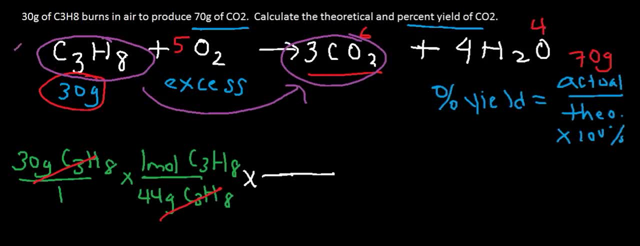 substance. you need to use the molar ratio, And the molar ratio it's a 1 to 3.. For every 1 mole of C3H8 that becomes CO2, you get 44. So you want to convert from moles of C3H8. 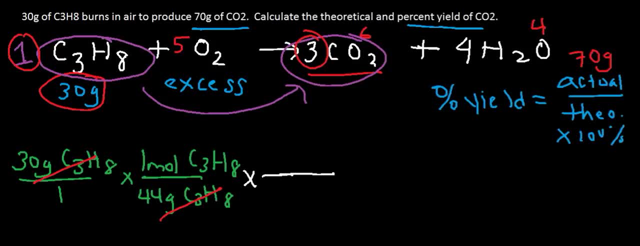 to moles of CO2.. Using this, you want to convert from moles of C3H8 to moles of CO2.. Entering the molar ratio, you want to convert from the mole here to the shuts, which is turning into 52, and you want to convert from moles of CO2 to moles of CO2, into moles of. 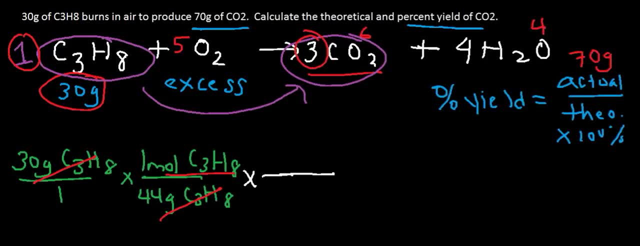 CO2.. When the moles of CO2, B and 0 curries, the moles of CO2 are produced And since we have moles of C3H8 on the top left, we need to put that on the bottom right so that they. 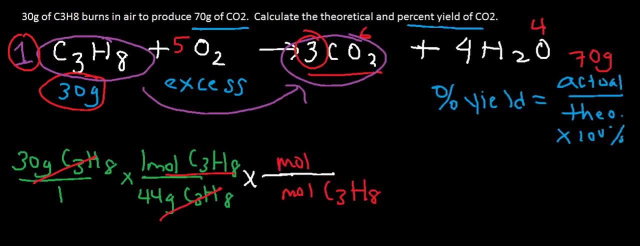 cancel And therefore the moles of CO2 will go on top. And then we simply add the numbers. There's a 1 in front of the C3H8, so we're going to put that here, And there's a 3 in. 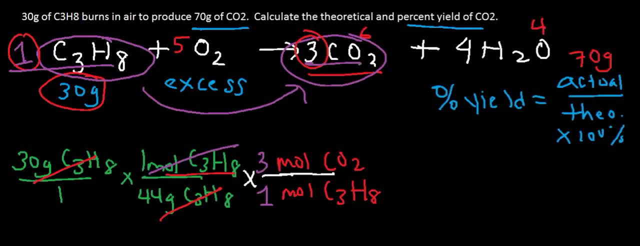 front of the CO2, so we'll put that there as well. So moles of C3H8, they cancel now Ulceration. the last step is to convert from moles back to grams. whenever you convert from grams to moles,